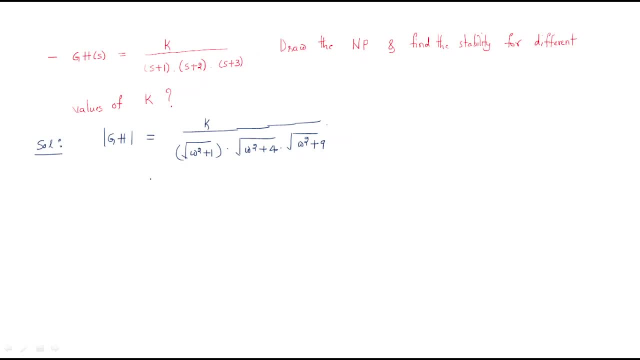 square plus 9.. This is the magnitude. and what about phase? We have to find out the phase Here. this is for 0 and for this is tan inverse of omega by 1, and for this tan inverse of omega by 2.. This is tan inverse of omega by 3.. Okay, right, So first we should find out. 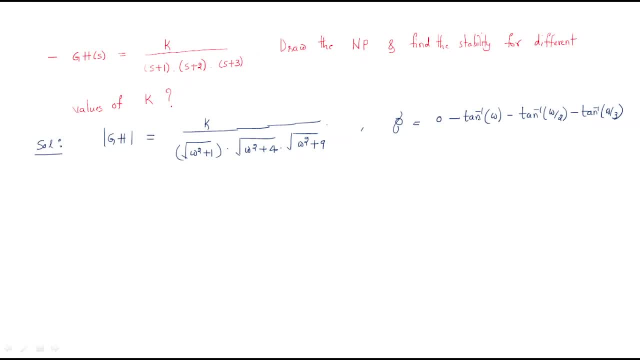 for we are getting magnitude values and phase values. First we should find out: at omega equal to 0, what is the at omega equal to 0.. First you find out for omega equal 0, what is the magnitude? Now we have? substitute it by this magnitude. substitute the omega values 0, K by this is 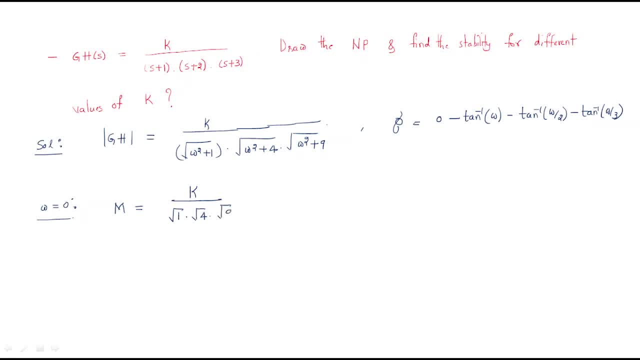 root 1 and this is the root 4 and this is the root 9.. so this is k by 1 into 2, into 3, so we will get magnitude 8.. frequency equal to 0 we were having. finally we will get the magnitude is k by 6. so k by 6.. So the Euro 1 is like that. So this is equal 10 k m ogni m over m, divided by 2, minus m by 1, divided by 1, multiplied to 0 by 15t, and we have the magnitude times 2. an inch x. Hamusiach u is 0. So we will get magnitude 8 of 4 is equal to 16 times 15.. So polygenitict g is like that: 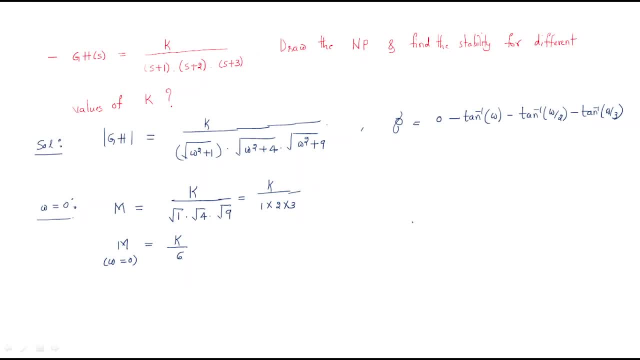 and, and so leave this thing. next we will go for draw the polar plot first for this. what is the polar plot we are getting here? so look at here here, this is the plot, this is general plot and this is the imaginary axis. and for this particular transfer function, the polar plot is like this: the polar plot is it. 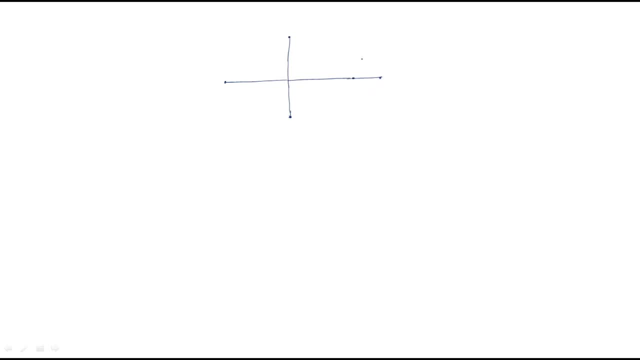 starts from here, for Omega equals 0 and Omega equals 0. this is the thing polar plot: Omega equals 0 and it will start at 0 and magnitude will be k by 6, so the plot is like this. so it's plot is start from here and 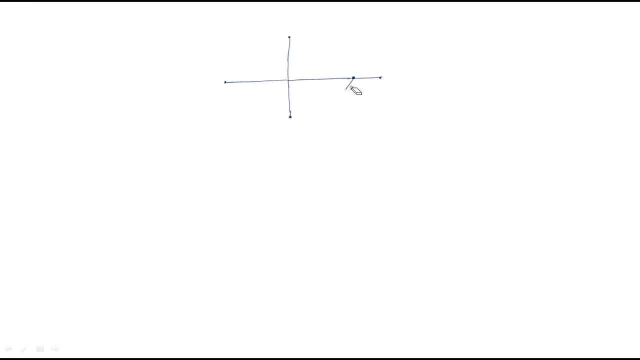 so we will modify it simply. the plot is: start from here and end with this point, and with here, this is Omega equal to 0 and at the Omega equals 0. what is the magnitude this plot? the magnitude of the plot is the k by 6. okay, so it start from. 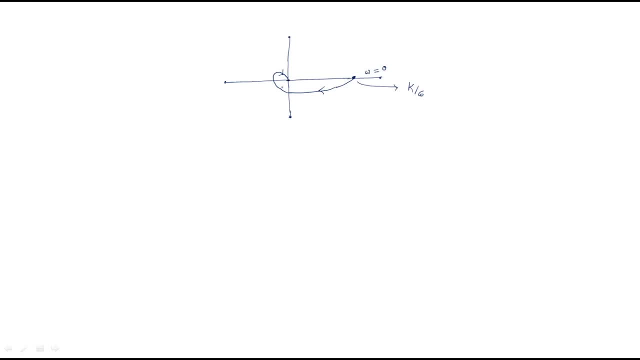 here and end with here. what is replica? so the replica is like this. so we should extend, we should just modify it, then it will clear. so it will be: start from here and and we'll touch it, touch this point and end with here: okay, this flow is like this. this flow is like this and end with here. so 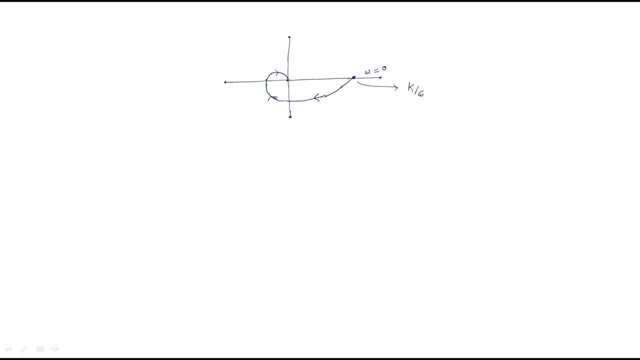 after reaching this point. so we should, you know, to get the polar night with plot, we should draw the replica of the polar plot. that's why the plot is exact replica is like this. so the exact replica is like this. so you start from here and right, so this will flow like: 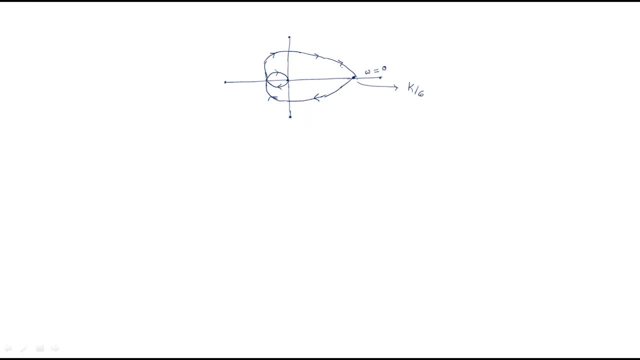 this. so you start from here and end with like this: start Omega equals 0 and it will omega equal infinite. after that replica is like this: okay, just observe the plot here and we will get. we were having, we are having here, omega equal 0, but we don't know what is. 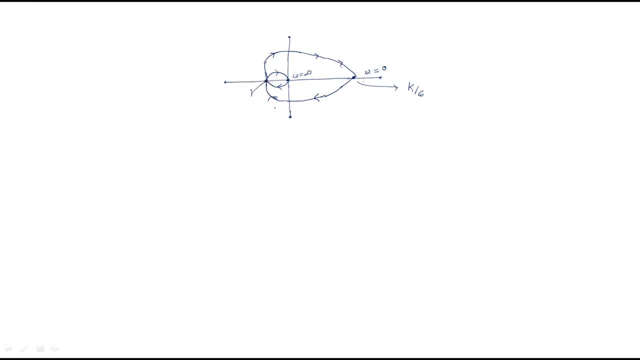 the omega at here. we don't know what is the omega at here, so we should find out what is the omega here. but you know that at this point the phase is minus 180. the phase is minus 180, so we will use that concept. the phase is minus 180, but what is the phase value? minus 180? the phase value is: 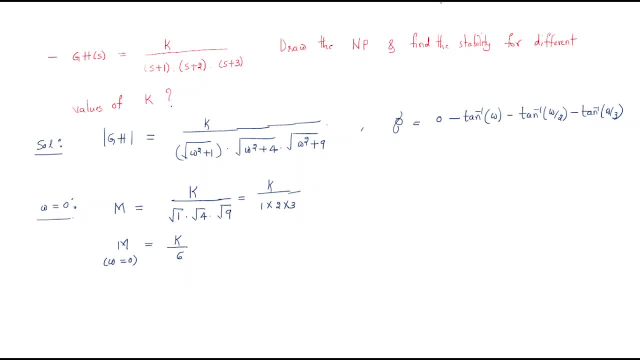 we will write here, so use this equation. the equation is tan inverse of omega, not tan inverse of omega minus tan inverse of omega. this is: and minus tan inverse of omega by 2 and minus tan inverse of omega by 3. why we are doing this we have to find out at phase of minus. 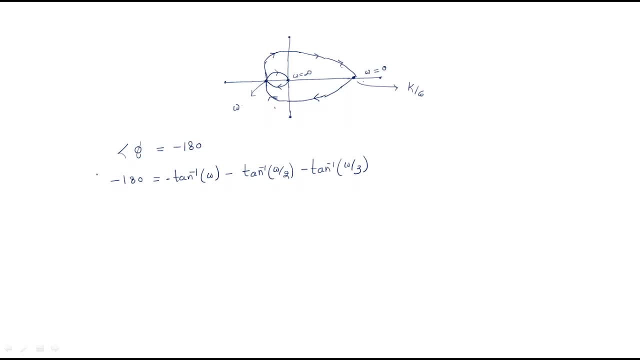 180. so if we are solving, we will get the omega value. so if you solve this by using a plus b principle, so the, if you solve this, 180 tan inverse of omega plus tan inverse of omega by 2, plus tan inverse of omega by 3, so it it looked. 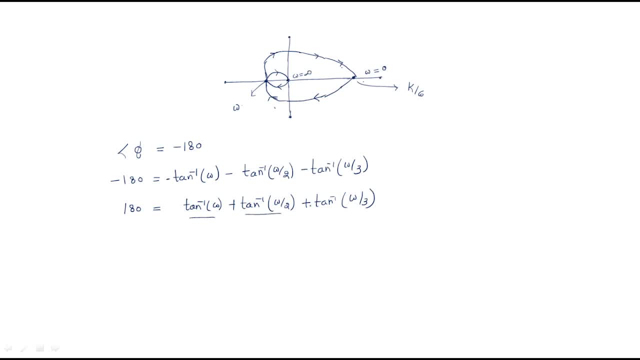 like tan inverse of a plus tan inverse of b. after the completion of this, you will apply again- this is the single- and apply for tan inverse of a and tan inverse of b. then you have. finally, if you solve this, we will get omega equaled 3.33 radian per second. you should do the, you should the, you should use the principle and solve. 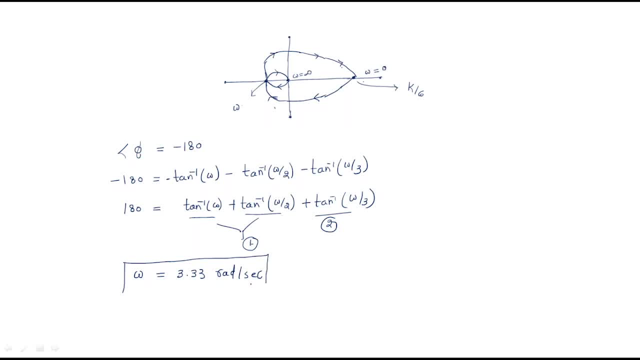 this, you will get the omega equaled 3.33 radian per second. so what is this meaning? at this, omega is 0 and it will reach this imaginary axis at omega equaled to 3.33. we will get, finally, 3.33 radian per. 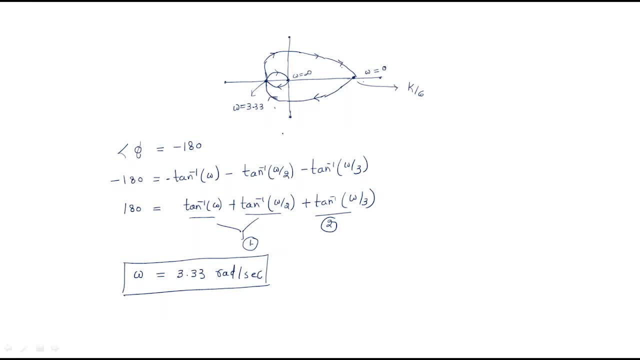 second: okay so, and we should find out the magnitude here. and what is the magnitude here? we should find out. so, at omega equaled at that point, at at the phase of minus 180, we will get. the frequency value is 3.33 radian per. 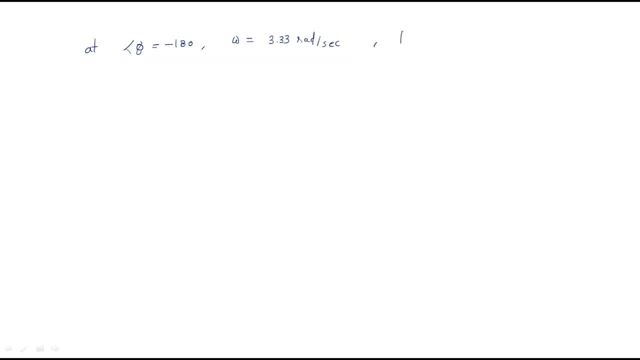 second, and at this we should find out the magnitude at omega equaled to 3.33. then what is the formula for magnitude gh at omega equaled to 3.33? already we write the magnitude here, so that's why we should substitute in this equation. we should substitute in this equation, in this equation if: 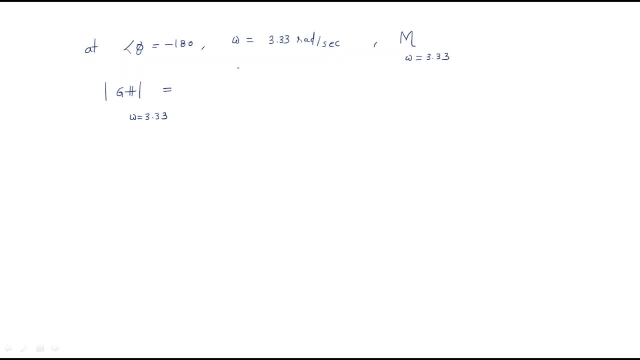 we substitute this, we will get in like this: 1 by under root of 3.33, whole square plus 1, and second is 3, point, sorry, separate thing. this is the 3.33 square plus 4, and what is the third third term is 3.33 square plus 9. okay so, and we have the magnitude is k, okay so by solving this, we 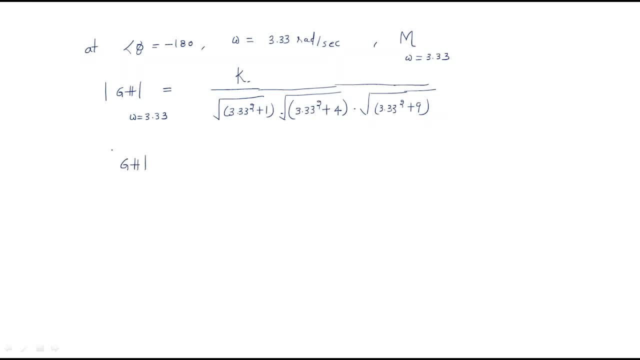 will get the magnitude at frequency equal to 3.33 radian per second is k by 60. so finally, we are getting the magnitude value at this. we are getting at this point. the magnitude value is k by 60. we have the k by 60 here, okay, but the question is, he is asking about stability. he is asking 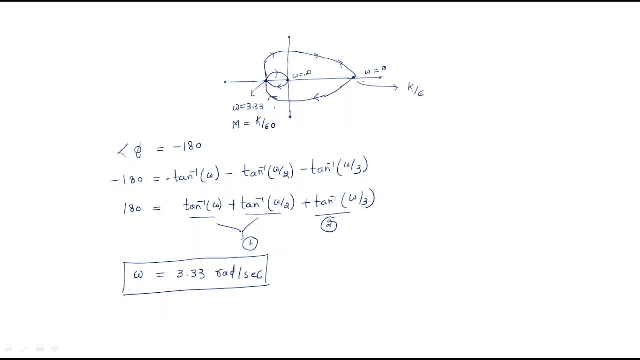 about stability. so, in order to get the stability first, where, where is the point of minus one, plus j- zero point? we don't know, maybe that point, maybe that point may be here or here, that point may be here. for example, assume we can use three cases. if the point is here: minus one, plus j- zero point is. 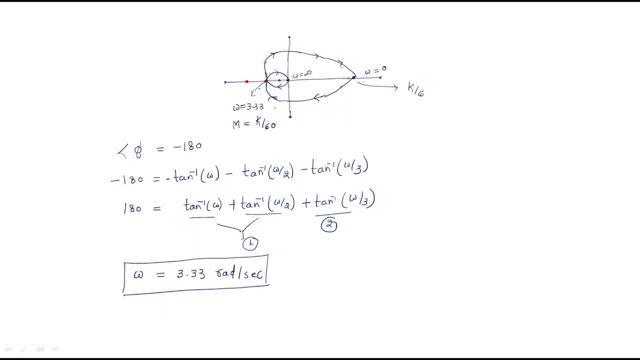 here or otherwise, here or otherwise. here, then we should find out stability, how the stability should be varied. we have to check it. so that is the condition. so that's why we will take here, that's why we'll write here, but we don't know. we don't know. 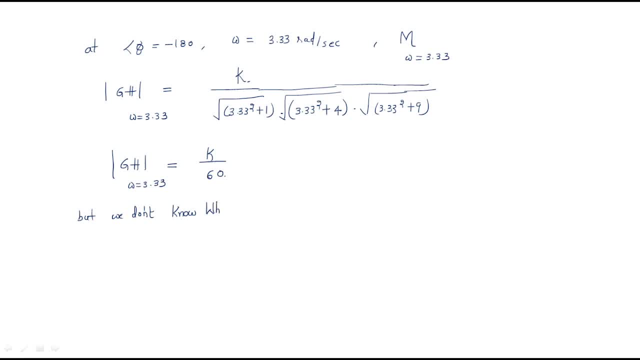 where is minus one plus j zero? where is minus one plus j zero? so we have but possibility cases are, but we have point of possibility cases are. we have three cases. first, case one, the case one. what is the case? one case one is, for example, here we have this point, for example, here we have minus one plus j zero. then then so for 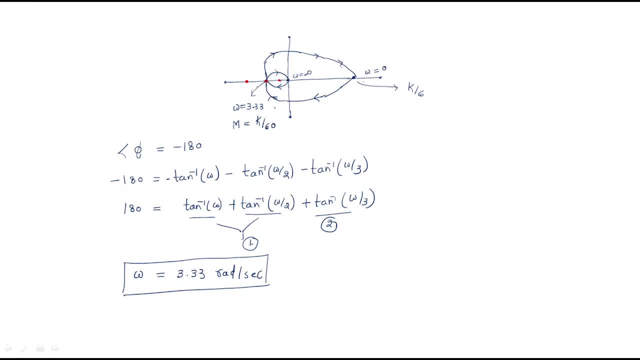 example. that means: how can we define this, this magnitude value, if, if it is here this, i can write like this: this is the right sign here, so this is the right sign here. so this is the right sign. this value is higher than this. so that's why I will write like this: if the k by 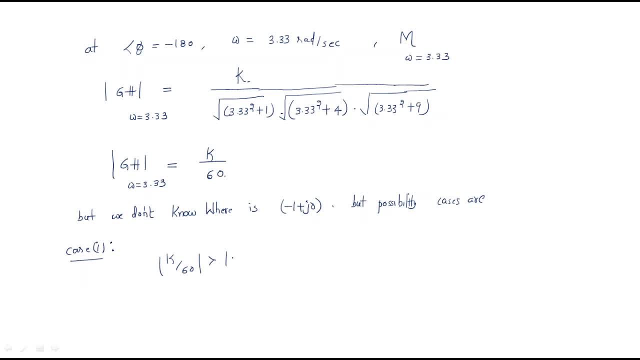 60 magnitude is greater than minus 1 plus j0. okay, so that's why we will get k by 60 is greater than 1. okay, so by using this, I will write k greater than of 60. this is the condition we are getting, but at this condition we will check the. 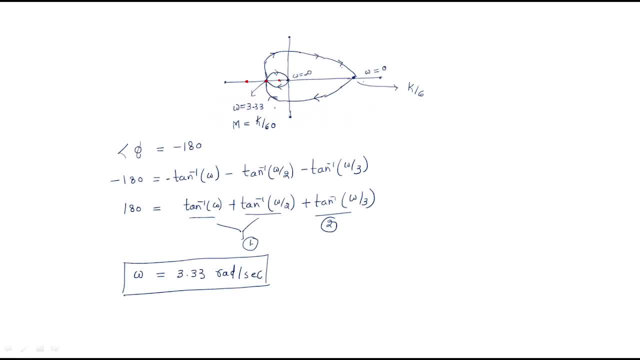 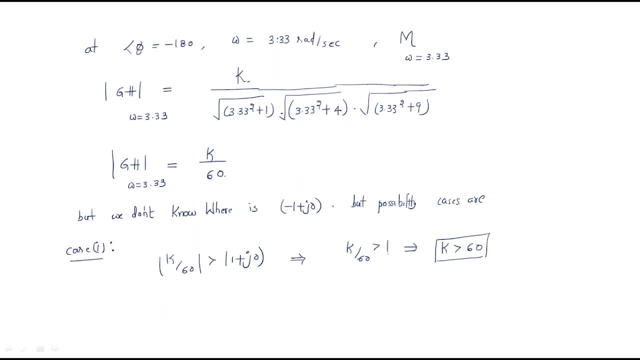 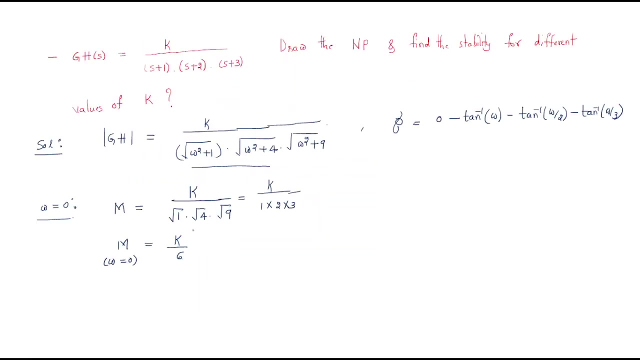 stability. so look at here in the integrity, what are the encirclements? one and two encirclements, because this is clockwise and this is also clockwise if there is. here the encirclements is, the two encirclements are clockwise, that's why minus two. and what is the? any open-loop poles is there for the system? 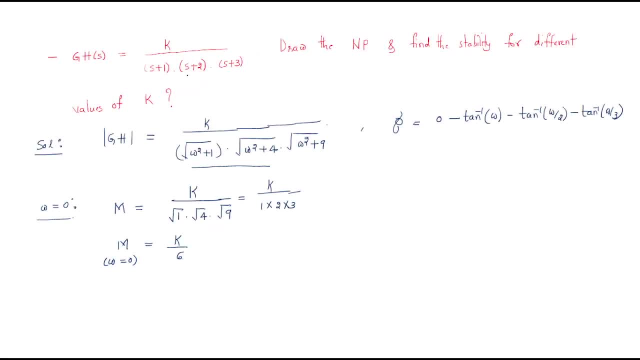 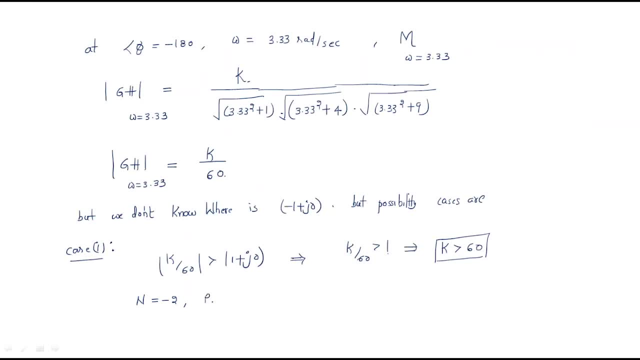 for the system. is there any right hand side pole in the open loop transfer function? no, that's why I will write: P plus value is 0, P plus value is 0 and we should find out open loop zeros, z plus value. so by using this we will get number of encirclements equal to P plus. 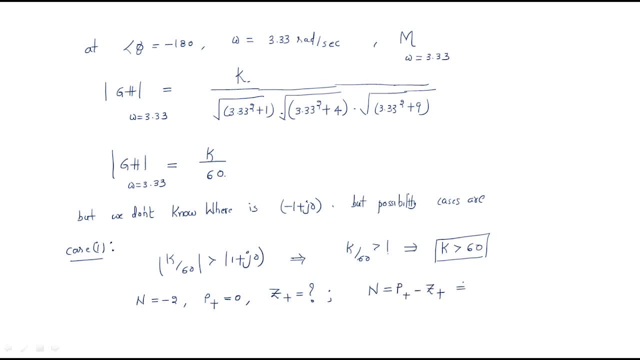 minus z plus what is P plus encirclements equal is minus 2 and 0 z plus equal to this. so close the loop. close the loop. right hand side poles are 2, so so this condition, at this condition, at k greater than 60 system is unstable. so the system. 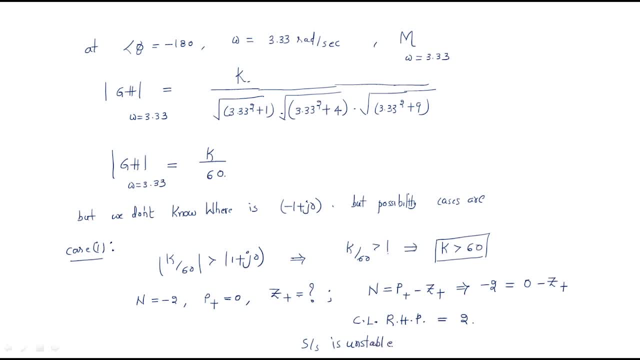 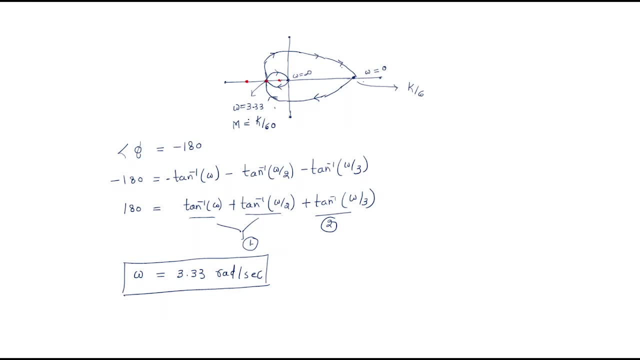 is unstable and we will use the second case. what is the second case here? if the point is here, if the minus 1 place j plus 0 is here, then both are same. this k by 60 and one value is same. so I will use the. 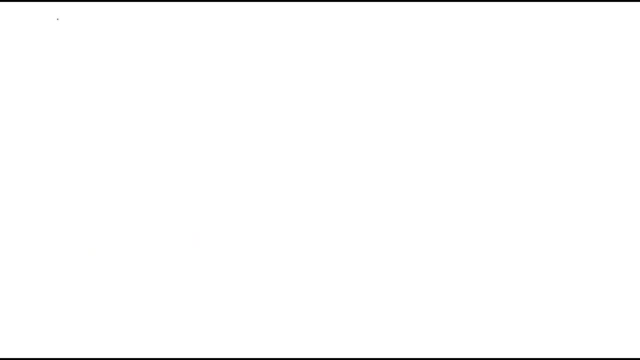 second case here, case to. I will use the case two. what is the case two? both are at the same point. k by 60, equal to a stand, should be 1. then K value equal to 60. if the k value is 60 here, if you put here: 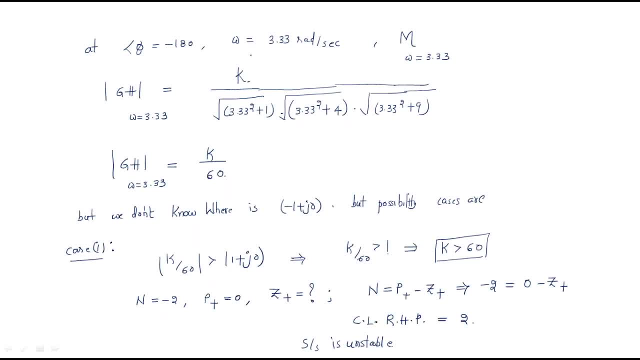 here there is no encirclements. there is no encirclements. that's why i will write: encirclements is 0 and poles are open. loop poles is 0, whatever z plus, we have to find out z plus equal encirclements. so we have to find out the z plus value. okay, so we know the encirclements. 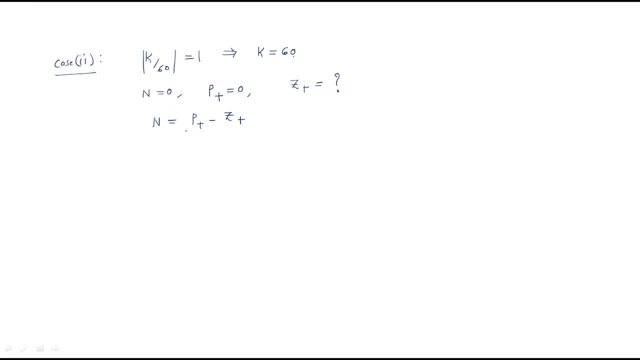 equal to poles minus open loop poles, minus closed loop poles, here 0 and this is the 0 and this is the z plus. so z plus equal to 0. that's why right hand closed loop poles are 0. therefore, at k equals 60. the system is stable. system. the system is stable. 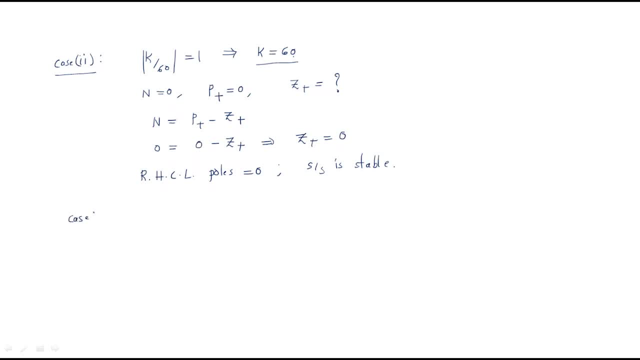 system system and we will use the case 3. what is the case 3 here here? if you observe the case 3, case 3 means if minus 1 plus j 0 is here. if minus 1 plus j 0 here, then what happened? minus 1 plus. 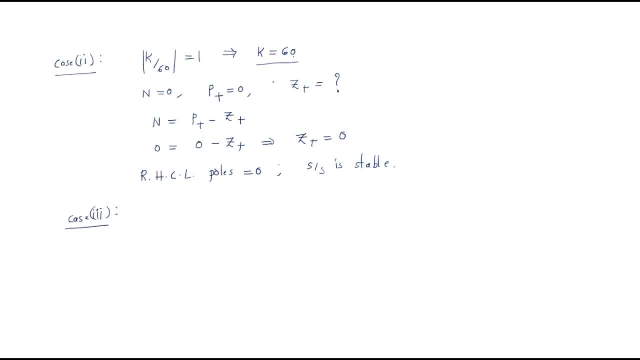 j, 0 magnitude is greater than the k by 60, so i will use that condition. that means so minus 1, plus j 0 magnitude is greater than the k by 60, so that's why this magnitude is 1 and k by 60. so at this condition, k value, so less than 60. 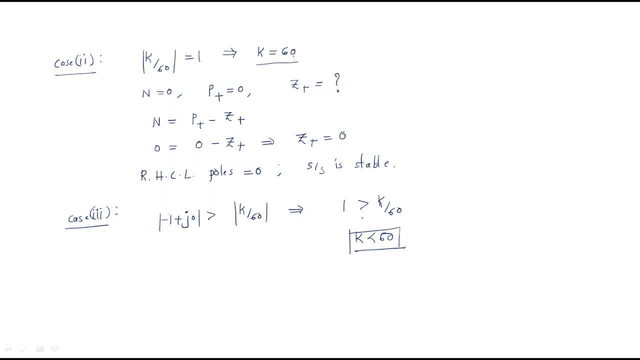 k value is less than 60. and at this condition- look at here what happened. at this condition, is there any encirclements? no, it doesn't have any encircles, so directly i will write: encirclements is 0, so any right hand side poles p.